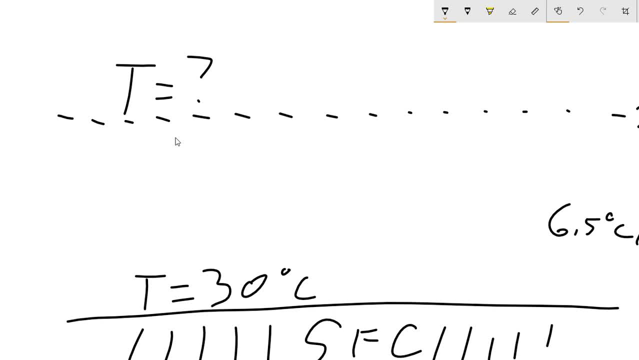 So how do we figure out the temperature at the 2 kilometer mark in the atmosphere? Well, we simply just do a little bit of math. So if we know that temperature changes every 6.5 degrees Celsius per 1 kilometer, 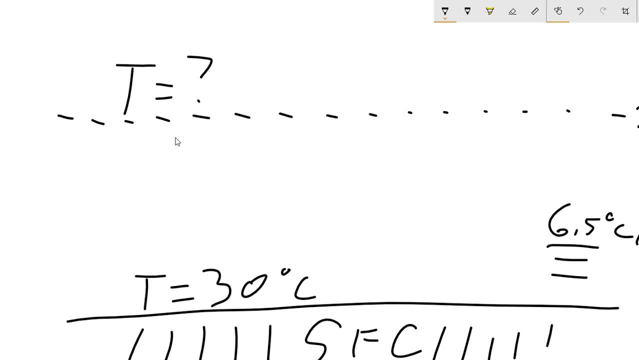 we know that if we go 2 kilometers, that temperature is not going to change once, it's going to change twice. So you can do 6.5 times 2, and that gives you 13.. So we know that temperature is now 13.. 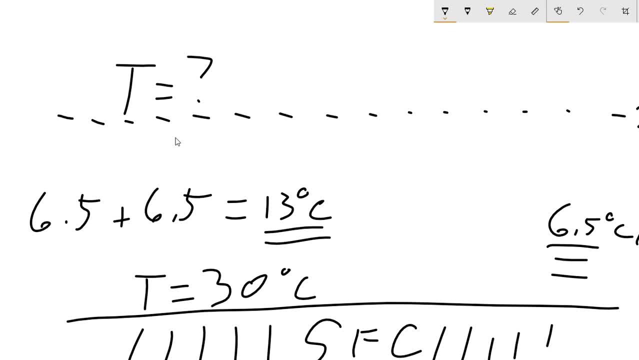 So we know that temperature is now going to change 13 degrees from the surface all the way up to 2 kilometers. All right, so now let's just clean this up real quick. Here's the surface And we know that temperature is 30 degrees here. 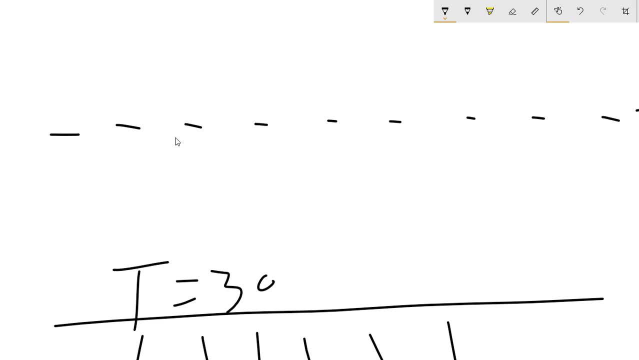 And we want to figure out the temperature here at 2 kilometers. So all we have to do- we know what the lapse rate is and we know that temperature is going to change. We'll call this delta. That's a way in the 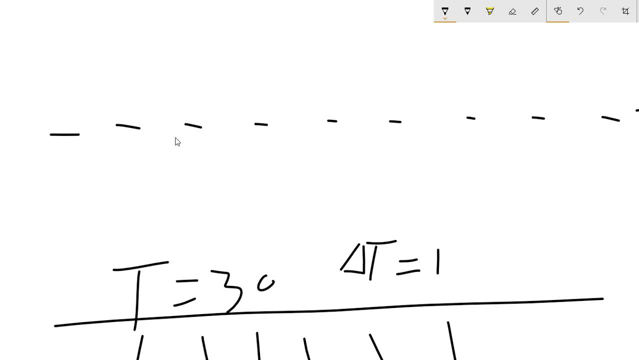 science community to denote change. So the change in temperature we know is going to be 13 degrees And you know that temperature should decrease the higher that we go up in altitude. So temperature here at 2 kilometers is going to be equal to the temperature at the surface, minus 13 degrees. 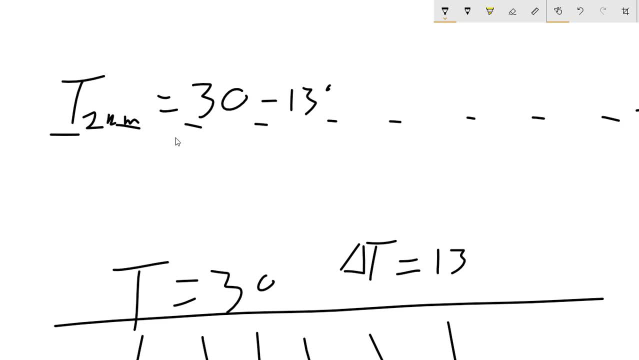 So that means that the temperature at 2 kilometers is actually 17 degrees Celsius, And that would be the answer here. So this is a way that you can use lapse rates. Now let's say we wanted to do it the other way. 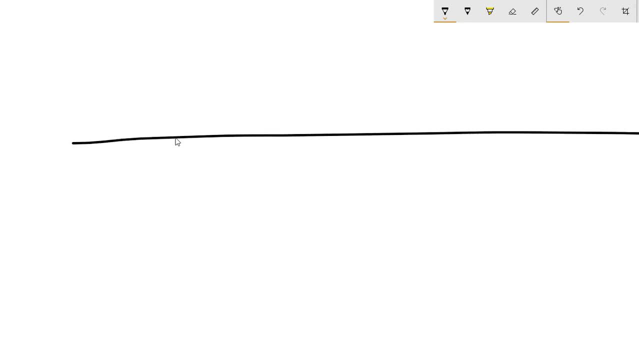 So let's say that we knew the temperature aloft And we say that the temperature at 2 kilometers or whatever it is, Let's say the temperature at 2 kilometers- was 15 degrees Celsius And we wanted to know the temperature at the surface here. 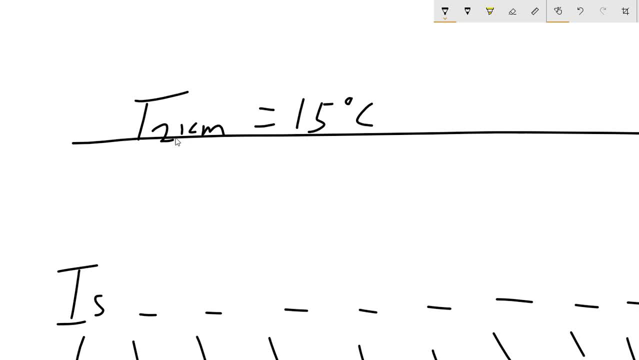 So we know that the temperature at the surface Right. We know that the lapse rate is going to change 6.5 degrees Celsius per kilometer And if this is 2 kilometers, Right, The distance between the top of the atmosphere, or this section of the atmosphere, to the surface. 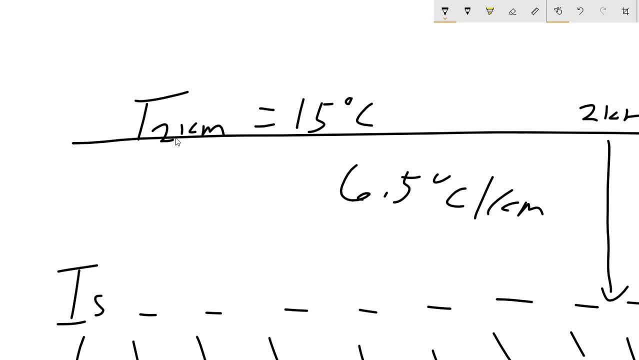 We know that temperature is going to change. what 13 degrees. We just did this, So the temperature at the surface Right Is just 15, plus We're adding because we're going towards the surface, The surface of the earth where it's warming- 15 plus 13,, which is what? 28 degrees Celsius. 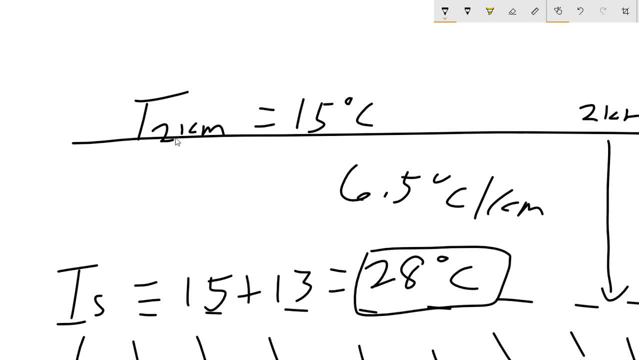 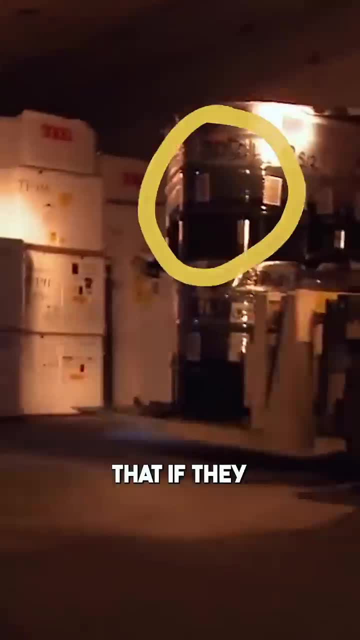 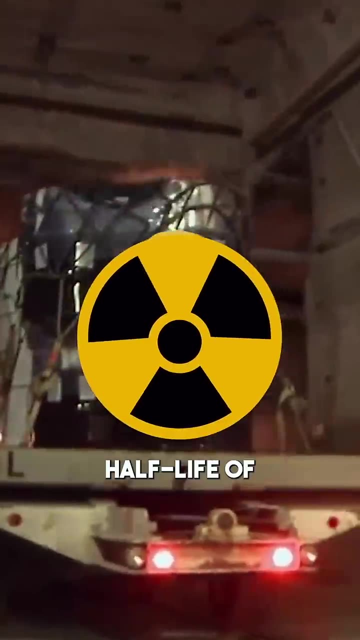 How could you communicate to humans 10,000 years in the future that if they open this box, they'll die? Inside this box is plutonium waste, which is very dangerous, and it has a half-life of over 24,000 years, so the contents will remain deadly for a very long time. One option is to use 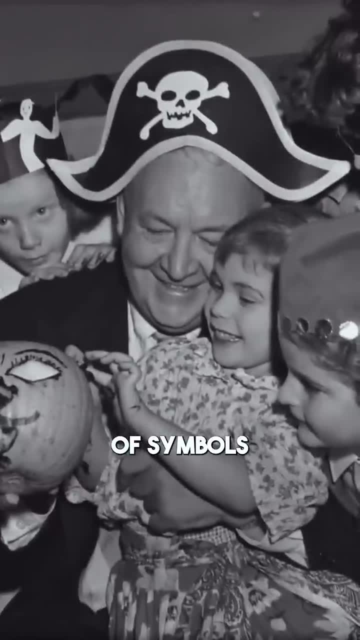 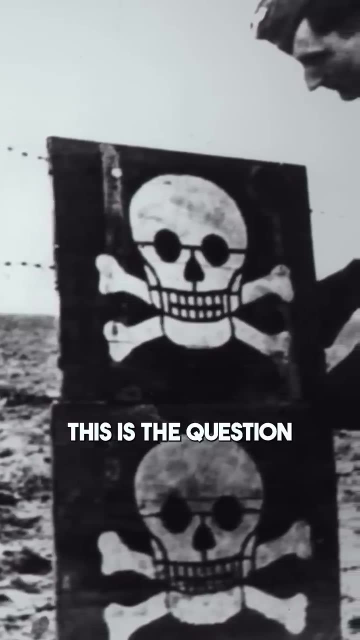 pictograms like a skull and crossbones, but the meaning of symbols drifts over time and the future. people might think that we're trying to tell them that this is where a pirate has buried his treasure. This is the question of nuclear semiotics. How can we communicate things to? 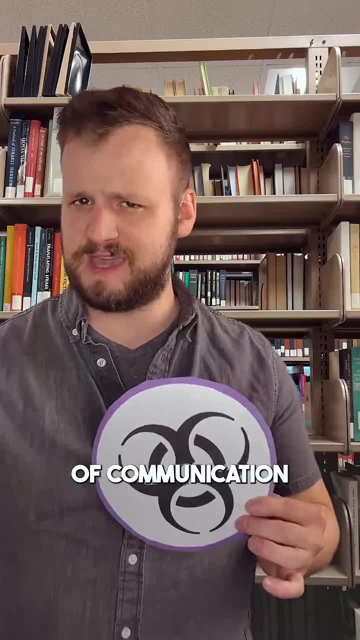 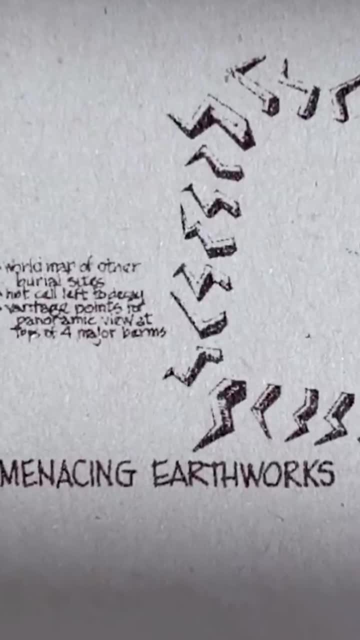 people in the future when we have no idea what system of communication they'll use. Another idea that we've tried is to use hostile architecture to like frighten people away from an area, but that could really backfire and end up arousing people's curiosity, Maybe the most. 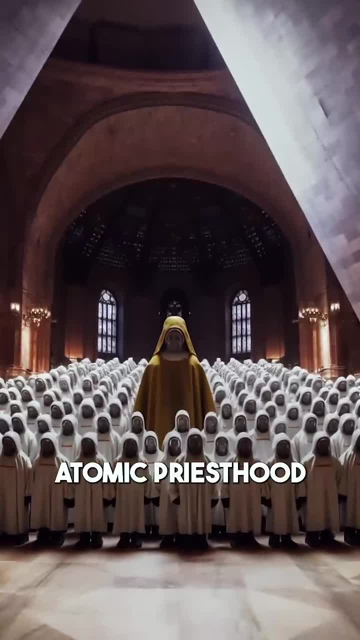 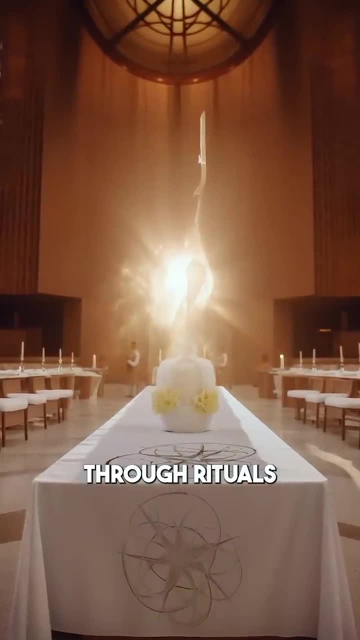 interesting idea came from a linguist who suggested we form an atomic priesthood, a council of about a hundred members who preserve the knowledge of the locations of nuclear waste through rituals and rituals. This is the question of nuclear semiotics. How can we communicate things? to people in the future when we have no idea what system of communication they'll use. Another idea is to use pictograms like a skull and crossbones, but the meaning of symbols drifts over time and the future. people might think that we're trying to tell them that this is where a pirate has buried. rituals and myths, but I could see how that could go poorly.